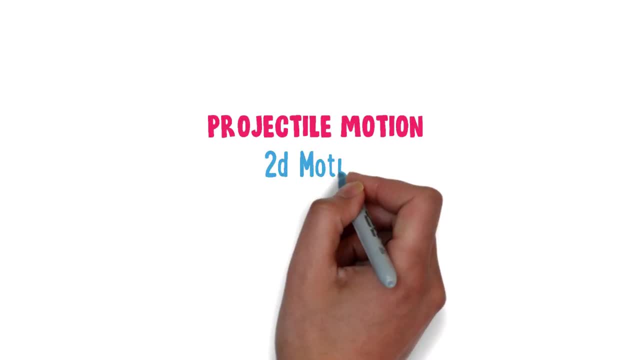 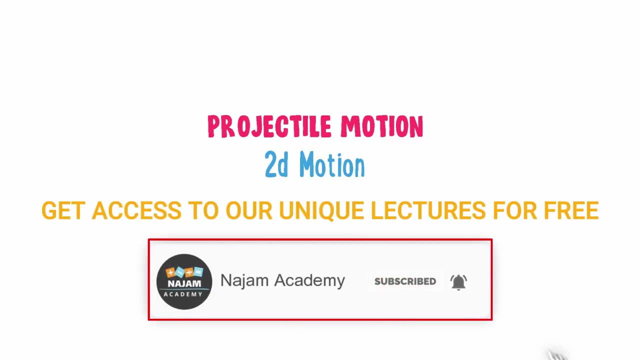 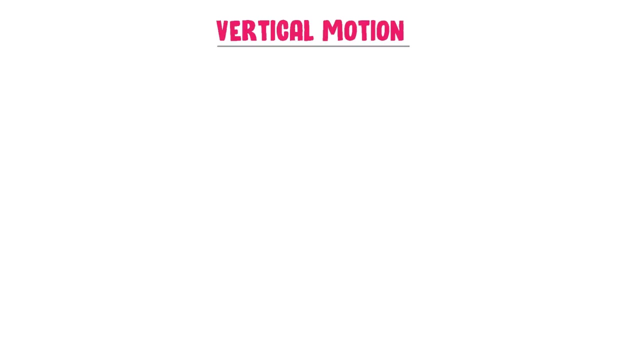 Understanding the Easy Concept of Projectile Motion and 2D Motion. Before starting the lecture, click on the subscribe button and get access to our 100 of unique and simple lectures for free. Firstly, let me teach you the vertical motion, which will make things super easy. For example, consider a ball present on the 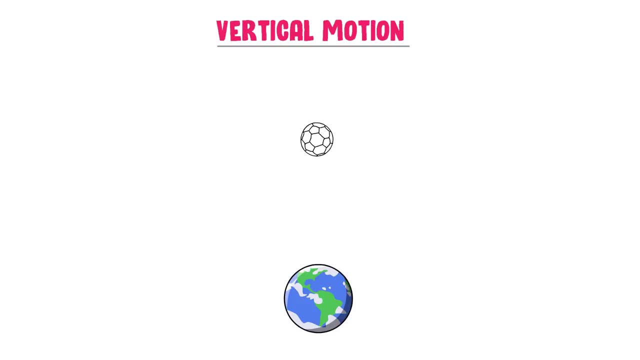 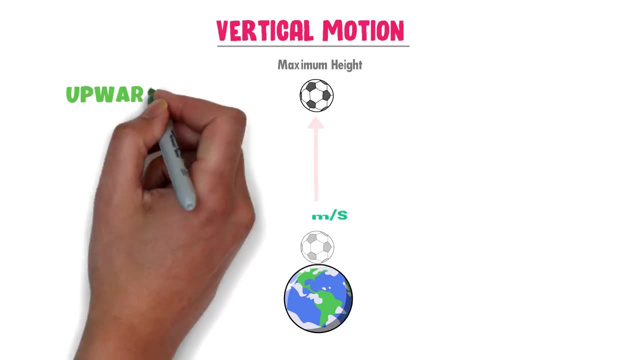 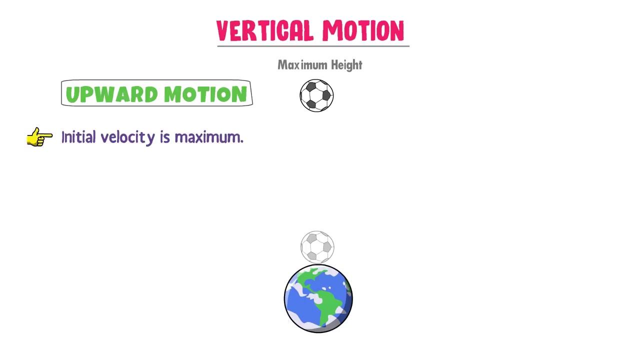 surface of the earth. Now you throw this ball in upward direction. Let the initial velocity of this ball is 10 m per second. Here let me discuss the upward motion of this ball. The first concept is that the initial velocity of this ball is maximum because when you throw the 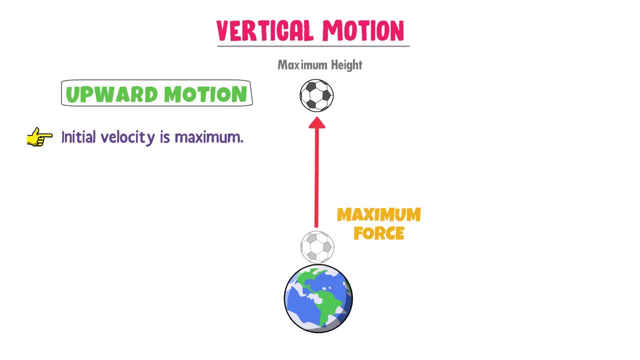 ball, you exert maximum force. The second concept is that the velocity decreases with the passage of time. as this ball gains height, It is because of the air resistance and gravity. The third concept is that velocity of this ball is 10 m per second. Let me discuss the upward motion of this. 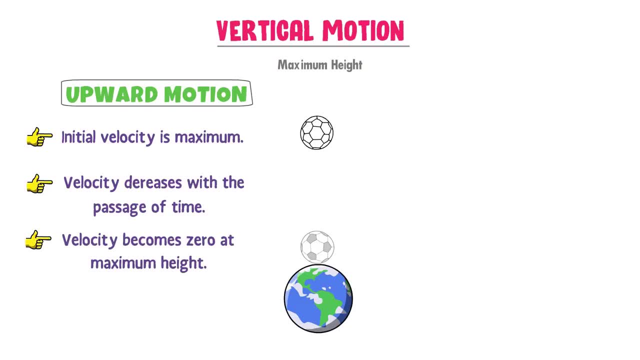 ball Here. let me also discuss the downward motion of this ball. We know that the velocity of this ball at maximum height is 0. So in the case of downward motion, the first concept is that the initial velocity of this ball is 0. The second concept is that velocity of this ball increases as it falls down. It is because of the downward force of this ball. 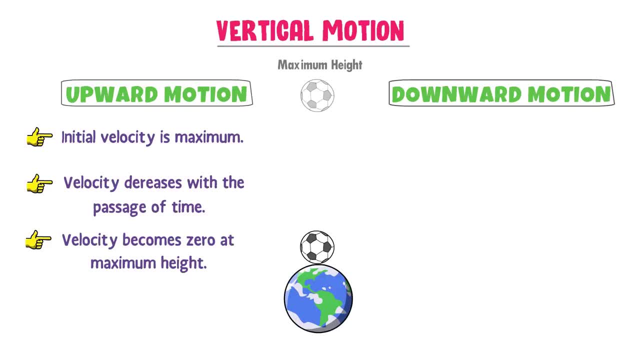 to discuss the downward motion of the ball. We know that the velocity of the ball at maximum height is zero. So in the case of downward motion, the first concept is that the initial velocity of the ball is zero. The second concept is that velocity of the ball increases as it falls. 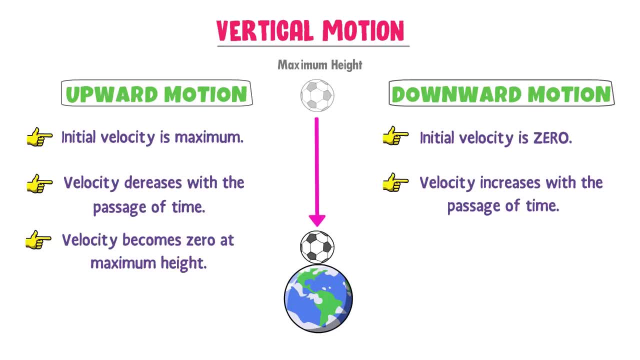 down, It is because of the downward force of gravity. The third concept is that the velocity of the ball is maximum just before hitting the ground. For example, its velocity may be 10 meter per second. Therefore, remember that in vertical motion, like upward motion, the initial velocity 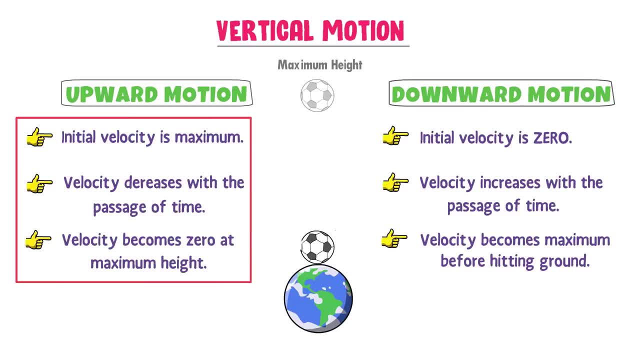 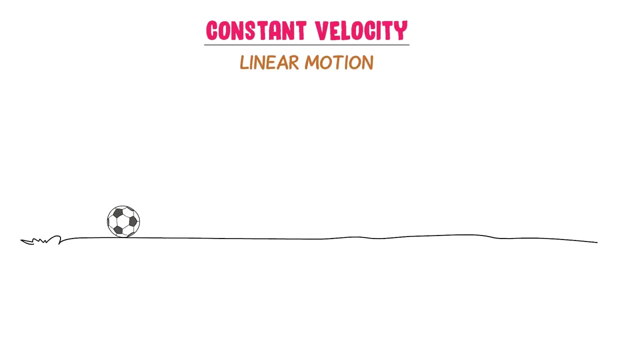 of the ball is maximum, but it decreases and becomes zero at maximum height. While in vertical motion, like downward motion, the initial velocity of the ball is zero, but this velocity increases and becomes maximum. Now you must also learn the constant velocity in linear motion. Consider a ball present on the 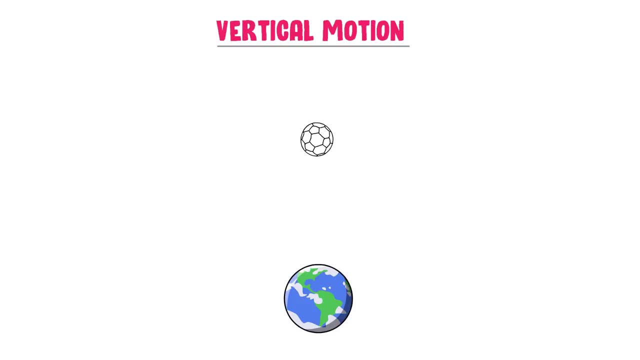 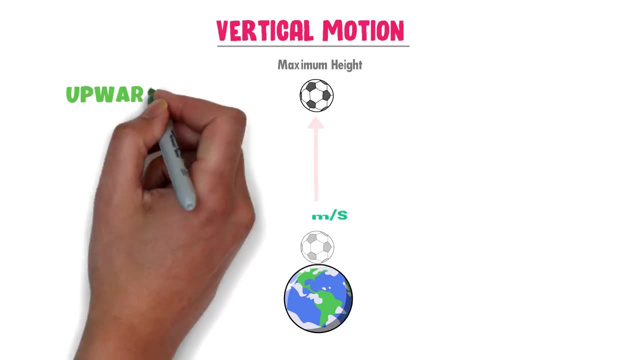 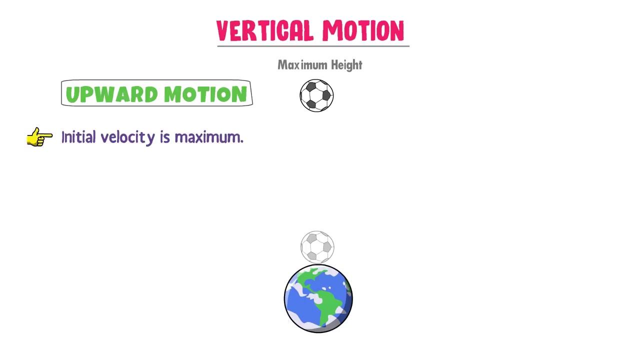 surface of the earth. Now you throw this ball in upward direction. Let the initial velocity of this ball is 10 m per second. Here let me discuss the upward motion of this ball. The first concept is that the initial velocity of this ball is maximum because when you throw the 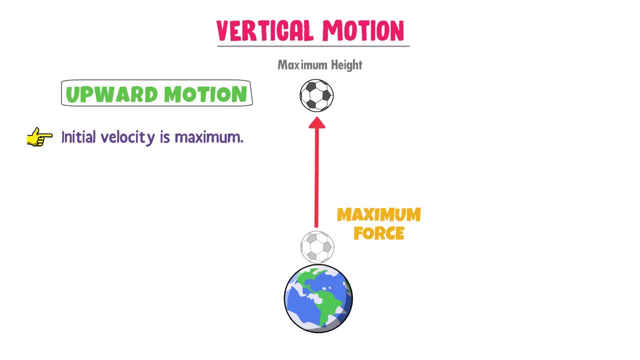 ball, you exert maximum force. The second concept is that the velocity decreases with the passage of time. as this ball gains height, It is because of the air resistance and gravity. The third concept is that velocity of this ball is 10 m per second. Let me discuss the upward motion of this. 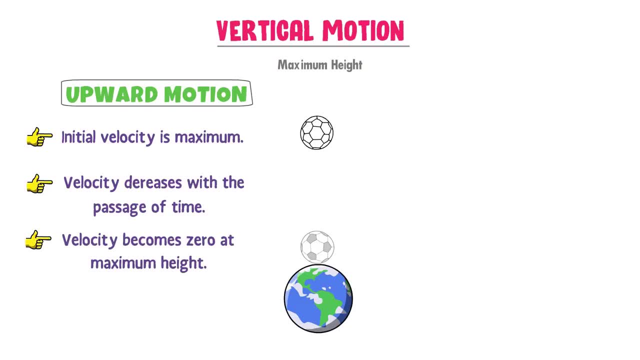 ball Here. let me also discuss the downward motion of this ball. We know that the velocity of the ball at maximum height is zero. So in the case of downward motion, the first concept is that the initial velocity of the ball is zero. The second concept is that velocity of the ball increases as it falls down. It is because of the downward force of this ball. 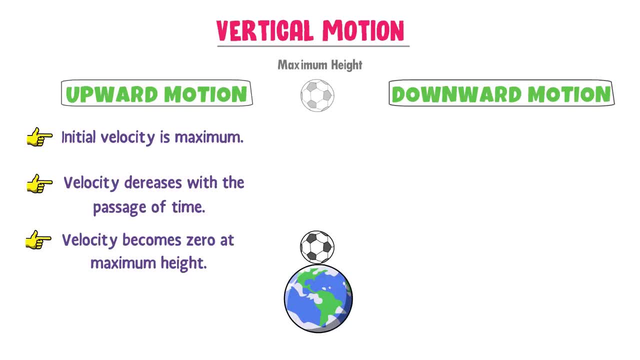 And the third concept is that the initial velocity of this ball is maximum. just before hitting Excess gravity peiful cool hitting the ground, For example, its velocity may be 10 m per second. Therefore, remember that in vertical motion, like upward motion, the initial velocity of the ball is maximum. 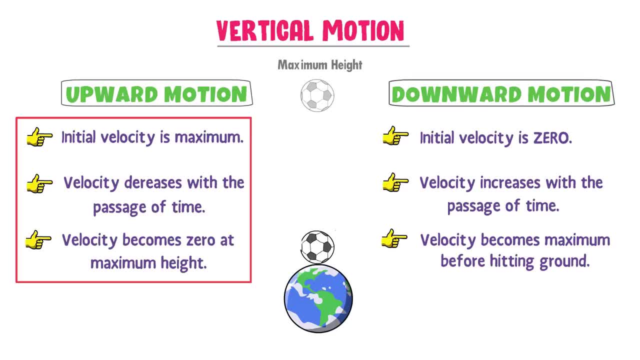 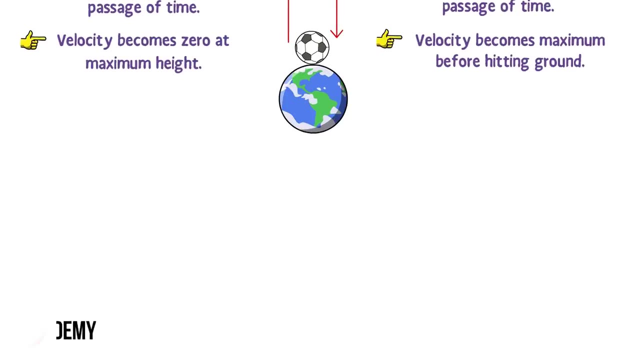 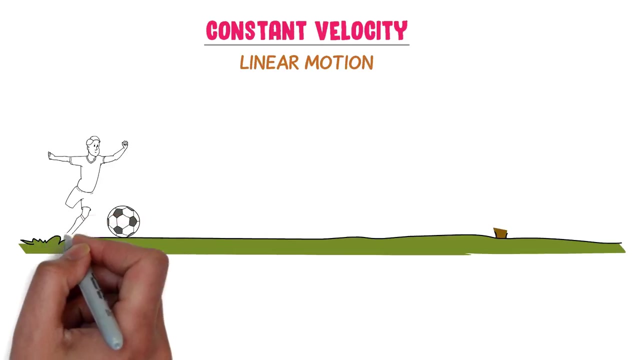 but it decreases and becomes zero at maximum height. While in vertical motion, like downward motion, the initial velocity of the ball is zero, but this velocity increases and becomes maximum just before hitting the ground. Now you must also learn the constant velocity in linear motion. Consider a ball present on the surface of a ground When you kick. 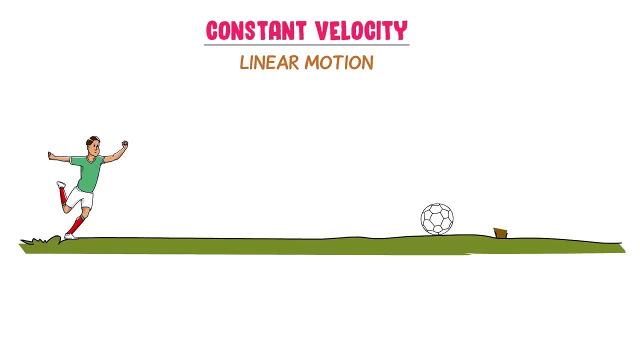 this ball. it starts moving. Let the initial velocity of this ball is 48 m per second. The ball covers some distance and finally it stops. This ball stops due to fractional forces like ground friction and air resistance. Now consider an ideal situation. 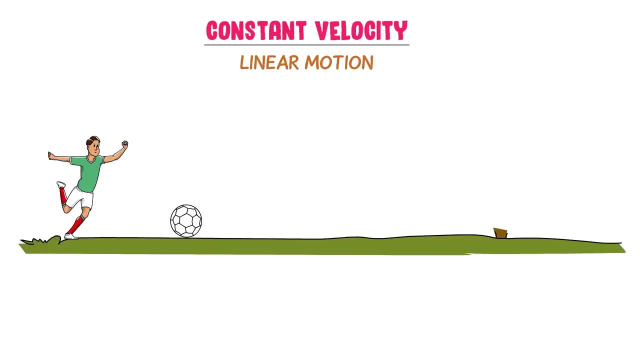 surface of a ground. When you kick this ball, it starts moving. Let the initial velocity of this ball is 48 meter per second. The ball covers some distance and finally it stops. This ball stops due to fractional forces like ground friction and air resistance. Now consider an ideal case. 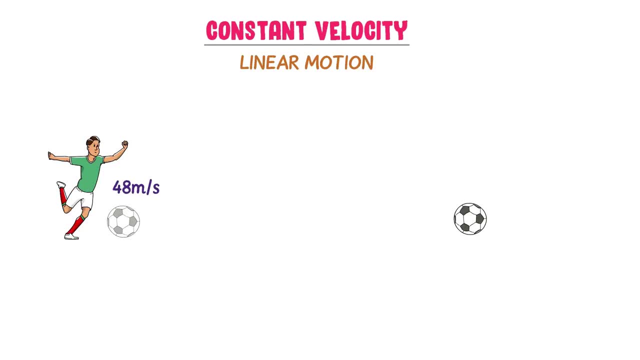 If we neglect the air friction and the ground friction, does the ball stop? The answer is no. No fractional forces mean that the ball will move with 48 meter per second at each and every point, forever. It is an ideal case which is not possible in real life. but we study. 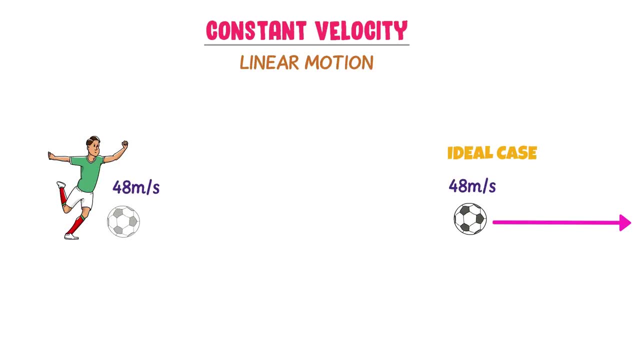 it only in physics. Therefore, we say that this ball is moving with constant velocity. Thus, remember that the initial velocity of the ball is zero and the initial velocity of the ball is 48 meter per second. Remember that, in absence of fractional forces, object moves with constant velocity. 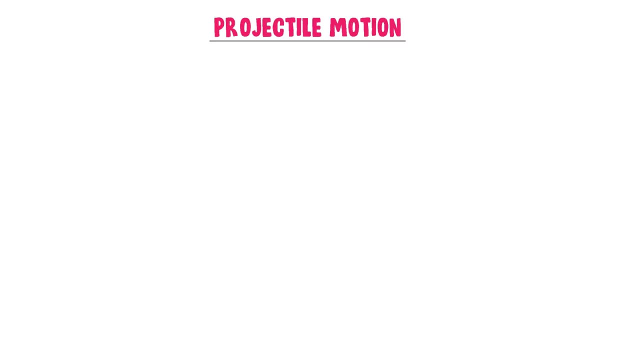 Now we can easily understand the projectile motion. Consider a ball. Let you kick this ball and it starts moving. We can see that the ball moves in parabolic path. I am interested to analyze the motion of the ball at this point. Initially, the ball is present here. 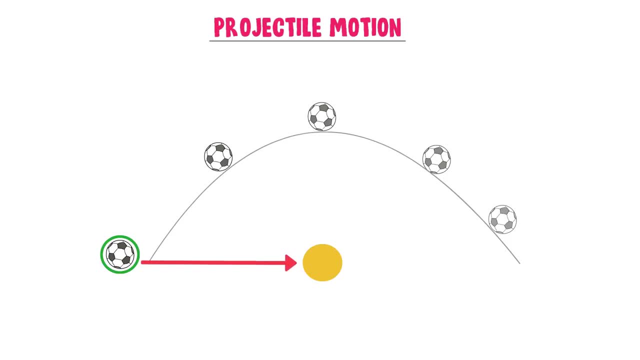 Horizontally. it has moved to this point, But the ball is not present here. It is present vertically at this point. With respect to its initial position, we say that the ball is moving in horizontal direction as well as in vertical direction. Let me repeat it. 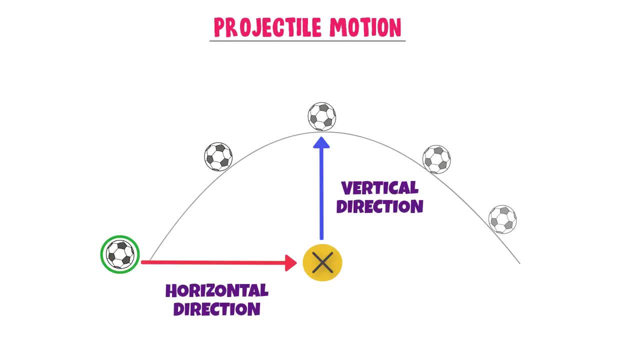 The ball is moving in horizontal direction as well as in vertical direction. In physics, such type of motion is called 2D motion, Because an object moves in x direction as well as in y direction. Therefore, we say that the projectile motion is 2D motion. Now consider that the initial velocity of the 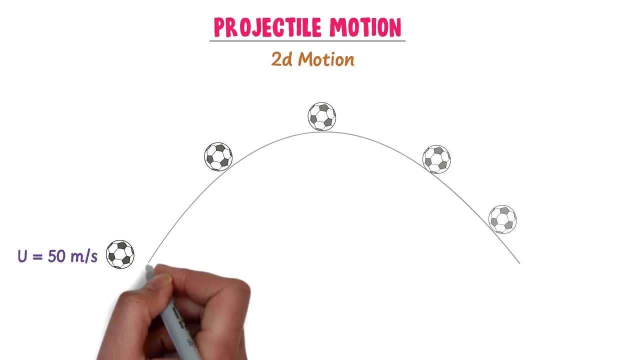 ball is: u is equal to 50 meter per second. Let the motion of the ball forms 20 degree angle with x axis. What about the horizontal velocity, ux, and vertical velocity? uy, Well, we know that ux is equal to 50 meter per second. Therefore, the horizontal velocity of the 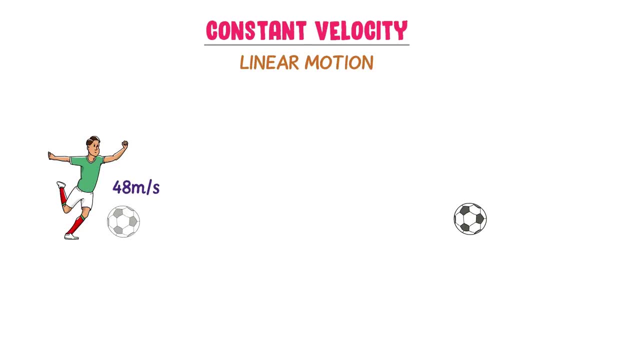 If we neglect the air friction and the ground friction, does the ball stop? The answer is no. No fractional forces mean that the ball will move with 48 m per second at each and every point, forever. It is an ideal case which is not possible in real life. but we study. 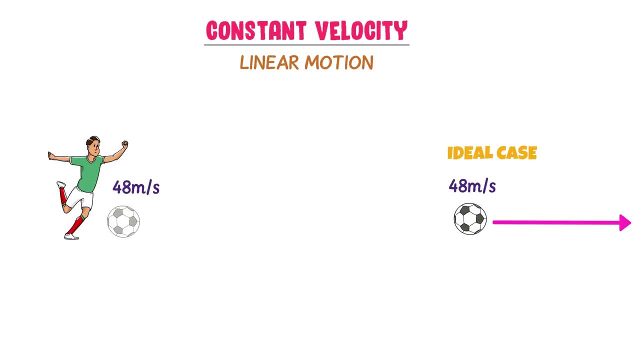 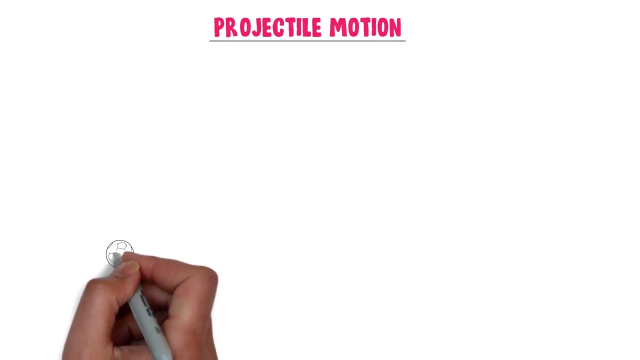 it only in physics. Therefore, we say that this ball is moving with constant velocity. Thus, remember that, in absence of fractional forces, object moves with constant velocity. Now we can easily understand the projectile motion. Consider a ball. Let you kick this. 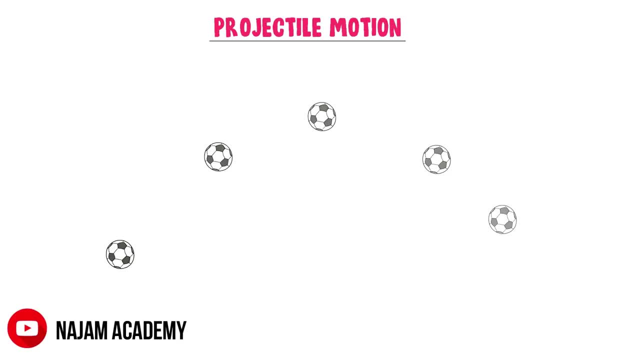 ball and it starts moving. We can see that the ball moves in parabolic path. I am interested to analyze the motion of the ball at this point. Initially, the ball is present here. horizontally it has moved to this point. But the ball is not present here. It is present. 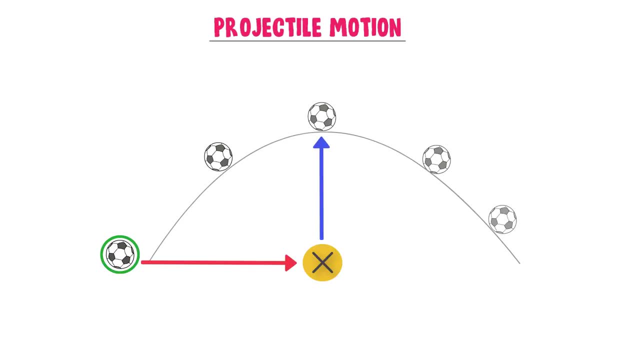 vertically. at this point, With respect to its initial position, we say that the ball is moving in horizontal direction as well as in vertical direction. Let me repeat it: The ball is moving in horizontal direction as well as in vertical direction. In physics, such type of motion is: 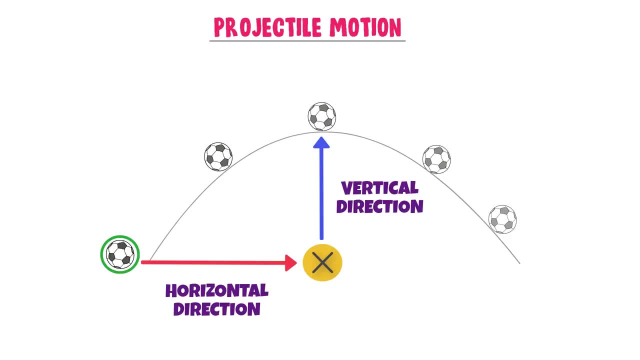 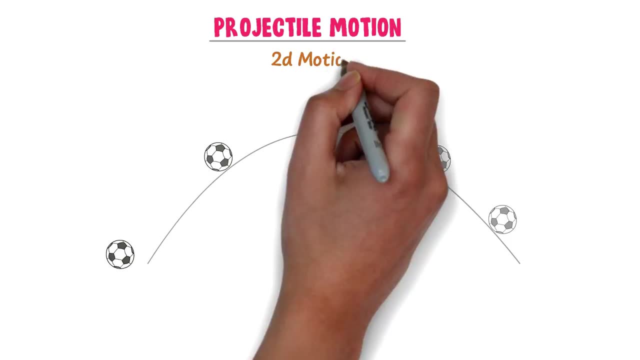 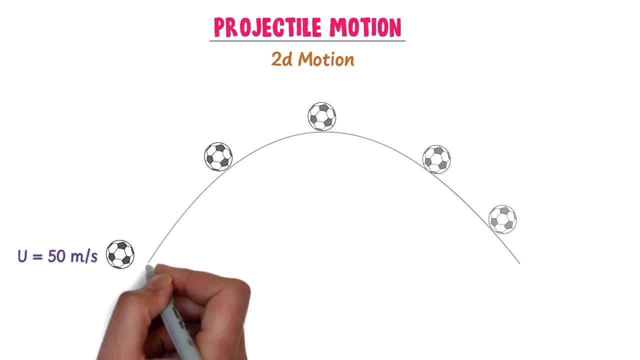 called 2D motion Because an object moves in x direction as well as in y direction. Therefore, we say that the projectile motion is 2D motion. Now consider that the initial velocity of the ball is u is equal to 50 m per sec. Let the motion of the ball forms 20 degree angle with x-axis. 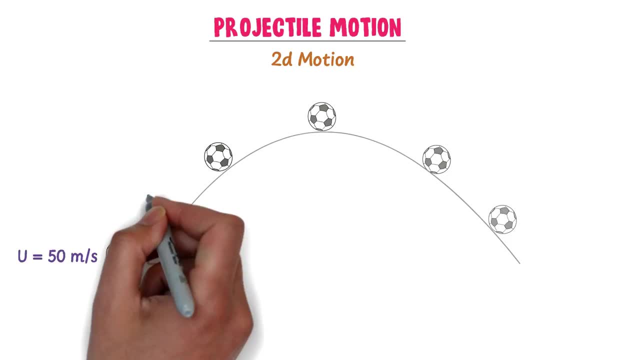 What about the horizontal velocity, ux, and vertical velocity, uy? Well, we said that the horizontal velocity tends to be 2d motion, So we can say that the velocity We know that ux is equal to u cos theta and uy is equal to u sin theta. 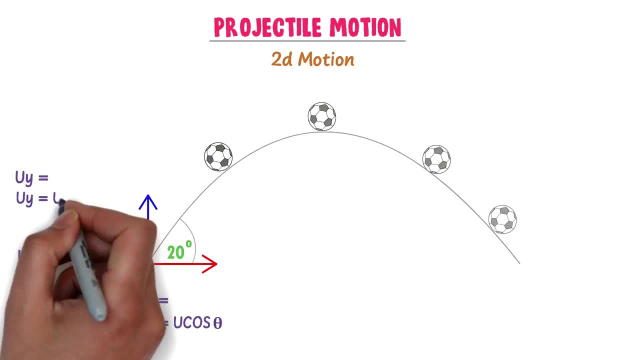 ball is equal to u cos theta and uy is equal to u sin theta. The value of u is equal to 50 and that of theta is equal to 20.. We get round about 47 meter per second. Thus the initial velocity of the ball in x direction is ux is equal to 47 meter per second. Similarly, 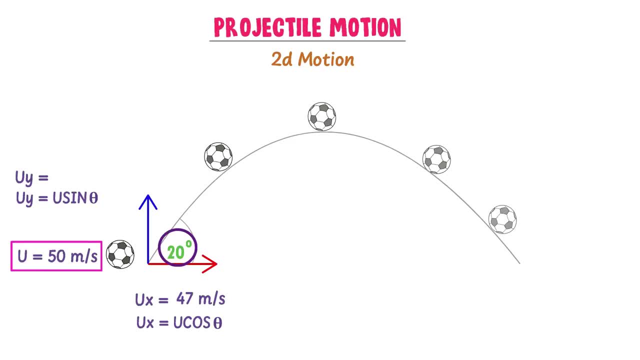 in the case of uy, put the value of u and theta, We get an entrance here, at the edge of the circle. here, If we made the path parallel to thequaling 20 degree of the quelle, we get that ux is equal to 70 meter per second. Thus the�를 velocity of the ball in y direction is ui. 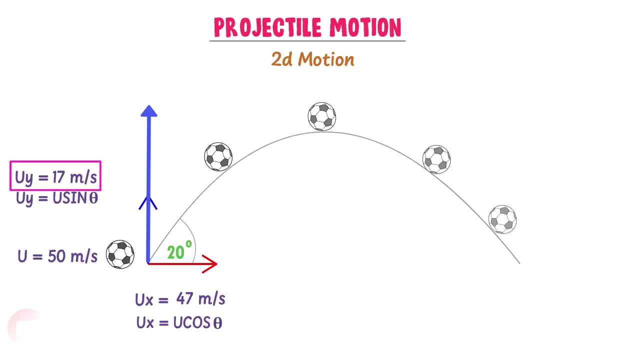 is equal to 17 meter per second. Neu, listen carefully. The ball is moving in the air, which means that along these surfaces where u theta and square external lines have a constant crochet may not be the same as the through surface surface, For examples. the ball experiences downward forces of gravity and further water resistance. 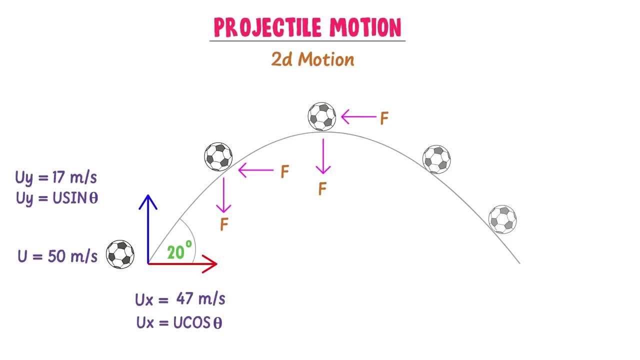 is being directed in this direction. and air resistance? At this point, the ball experiences force of gravity and air resistance As an ideal case. I neglect the air resistance on the ball at this point. I also neglect air resistance at this point, and I again neglect air resistance at this point. Let me ask you: 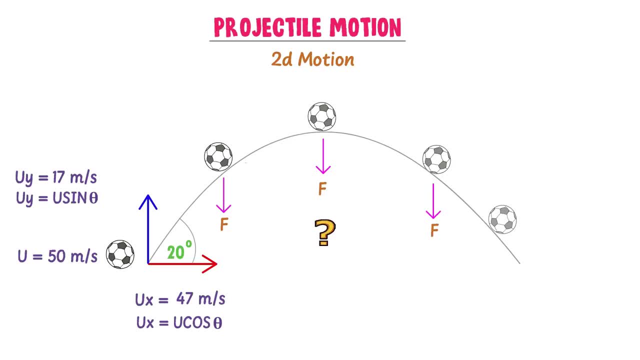 how many forces are acting on the ball? Well, the answer is 1. Only one force, the downward force of gravity, is acting on the ball. Therefore, note it down that only gravity acts on projectile. It means that there is no horizontal force acting on the ball. Thus, the initial velocity of the 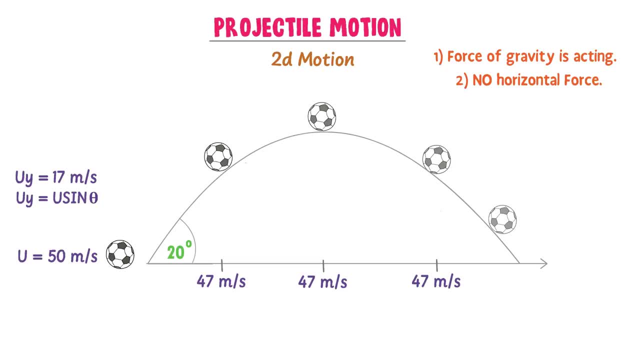 ball along x-axis would be 47 m per second at each and every point. We say that the ball moves with constant velocity in x-axis direction. It is because no force is acting along x-axis. Now what about the velocity of the ball in vertical direction? Well, the initial velocity 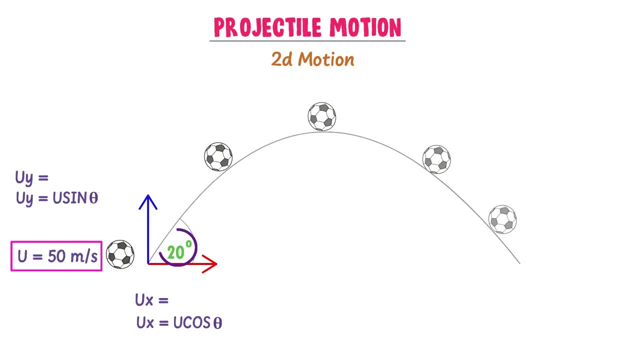 The value of u is equal to 50 and that of theta is equal to 20.. We get round about 47 m per second. Thus the initial velocity of the ball in x direction is ux is equal to 47 m per second. Similarly, in the case of uy, put the value of u and theta. 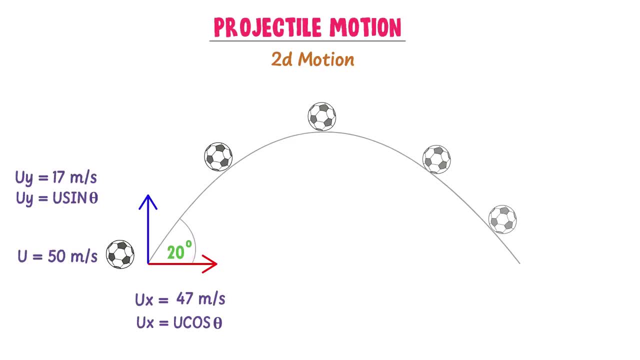 We get uy is equal to 17 m per second. Thus the initial velocity of the ball in y direction is uy is equal to 17 m per second. Now listen carefully. The ball is moving in the air. The ball experiences two types of forces. 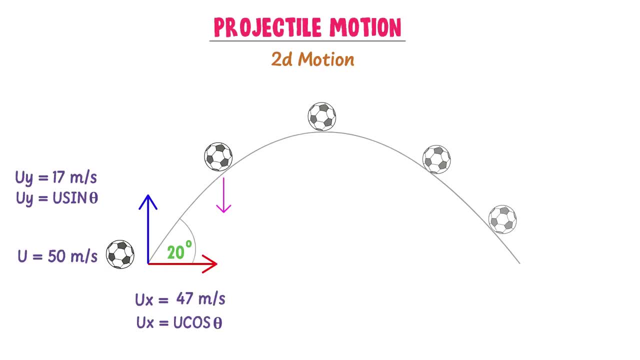 For example, at this point, the ball experiences downward force of gravity and air resistance in this direction. At this point, the ball experiences downward force of gravity and air resistance in this direction. At this point, the ball experiences force of gravity and air resistance in this direction. 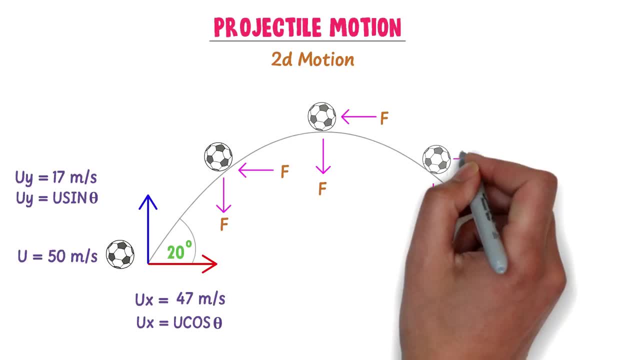 At this point, the ball experiences force of gravity and air resistance As an ideal case. I neglect the air resistance of the ball at this point. I also neglect the air resistance at this time, and I again neglect the air resistance at this point. 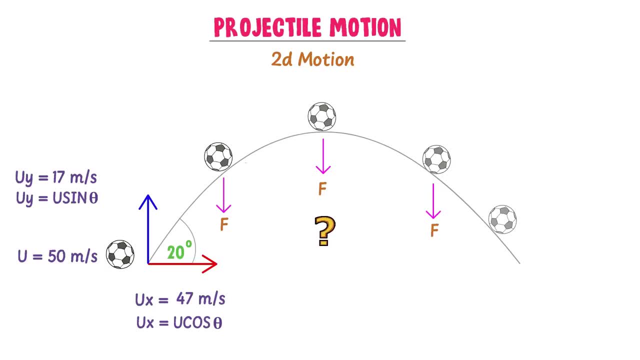 Let me ask you how many forces are acting on the ball. Well, the answer is one: Only 1. number one force, the downward force of gravity, is acting on the ball. Therefore, noted down that only gravity acts on projectile. It means that there is no horizontal force acting on the ball. 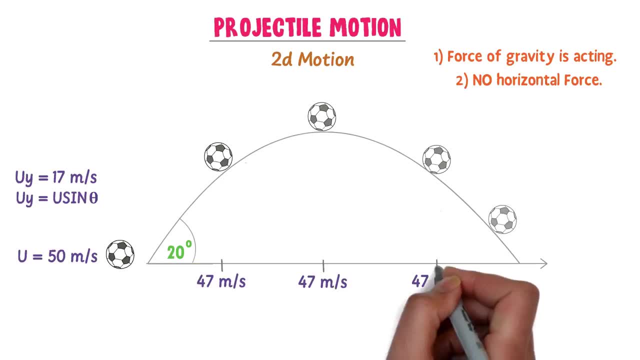 Thus the initial velocity of the ball along x-axis would be 47 m per second. at each and every point We say that the ball moves with constant velocity in x-axis direction. It is because no force is acting along x-axis. Now what about the velocity of the ball in vertical? 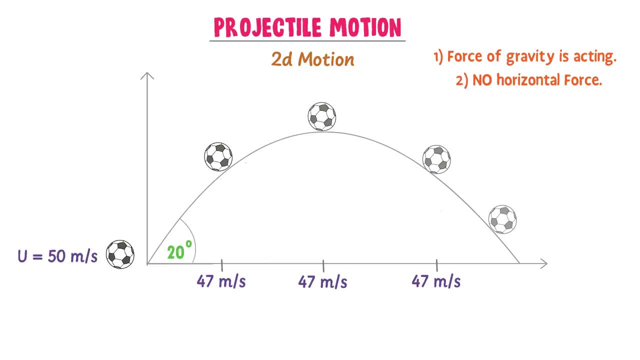 direction. Well, the initial velocity of the ball in y-direction is 17 m per second. But as the ball gains height, its velocity decreases with the passage of time. For example, at this point is 9 m per second, at this point is 5 m per second and finally the velocity of the ball becomes zero. 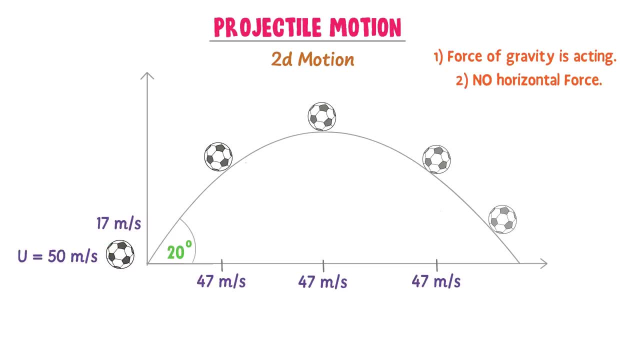 of the ball in y-direction is 17 m per second. But as the ball gains height, its velocity decreases with the passage of time. For example, at this point is 9 m per second. at this point is 5 m per second. At this point, the velocity of the ball is 9 m per second. At this point, 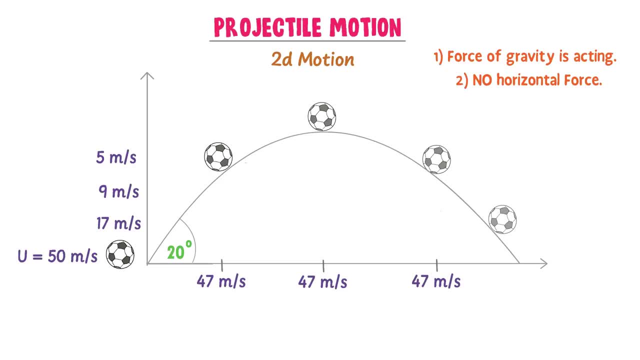 the velocity of the ball is 9 m per second. At this point the velocity of the ball is 5 m per second And finally the velocity of the ball becomes 0.. If you do not understand that why velocity of the ball decreases, then it is because ball wants to move in upward. 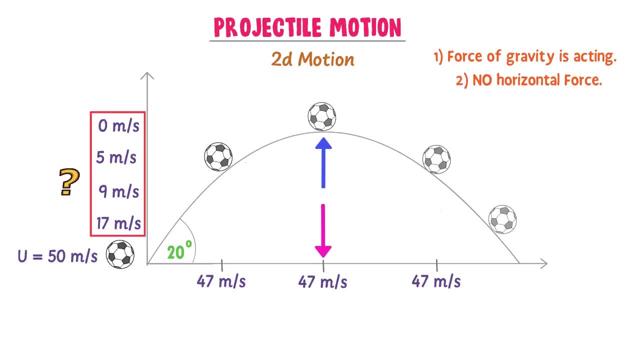 direction, but the gravity is pulling it in downward direction and thereby decreasing its velocity. Until now we have learned that in projectile motion, an object like ball moves with constant initial velocity along horizontal direction. Now let me analyze the motion of the projectile or the ball at each and every point, which. 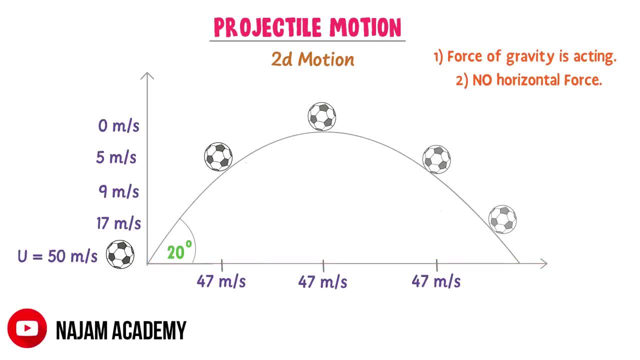 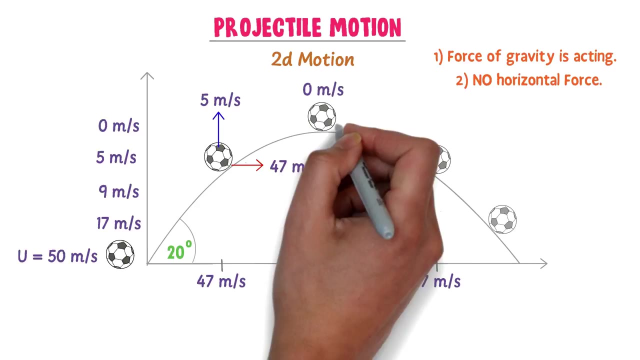 will further strong your concepts. For example, at this point the vertical motion of the ball is 5 m per second and its horizontal motion is 47 m per second. At maximum height, the vertical motion of the ball becomes zero, but the horizontal motion of the ball is. 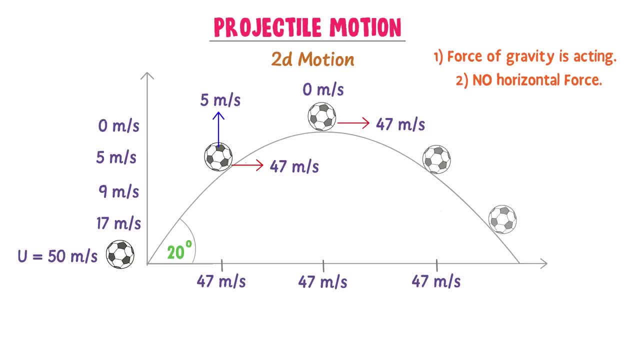 still 47 m per second. Remember that at maximum height the motion of the ball is not zero, because the ball still moves with 47 m per second in horizontal direction. Only the y-component, or vertical component, of motion is zero. Now the ball will start falling down At this. 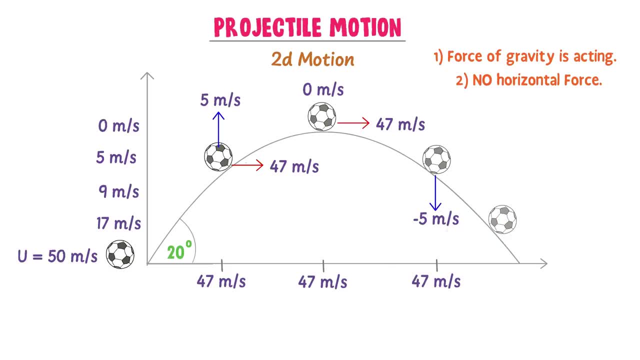 point the vertical velocity of the ball is 0.. At this point the vertical velocity of the ball is negative 5 m per second and its horizontal velocity is 47 m per second. And at this point the vertical velocity of the ball is negative 17 m per second and its horizontal 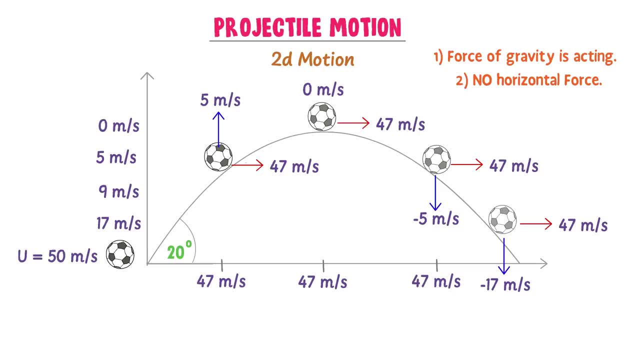 velocity is 47 m per second. Remember that negative sign doesn't indicate the smaller value, it only indicates the opposite direction of the ball. Thus we can analyze that as expected. Because of percent quantity of the velocity of the ball, the velocity of the ball varies. 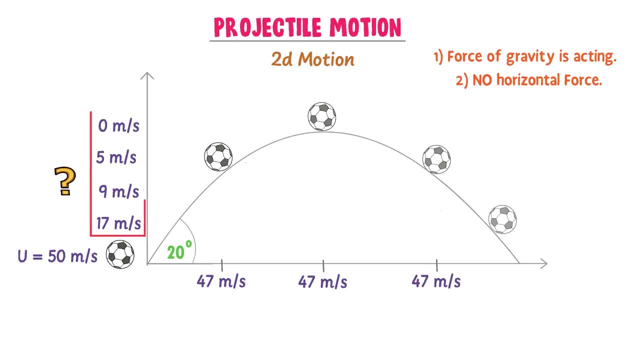 If you do not understand that why velocity of the ball decreases, then it is because ball wants to move in upward direction, but the gravity is pulling it in downward direction and thereby decreasing its velocity. Until now we have learned that in projectile motion, an object like ball 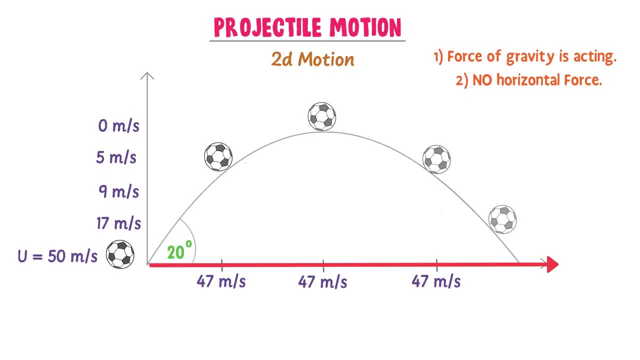 moves with constant initial velocity along horizontal direction or x-axis. While the velocity of the ball in vertical direction is 0.5 m per second, the velocity of the ball in vertical direction or y-axis decreases with the passage of time. Now let me analyze the motion of the. 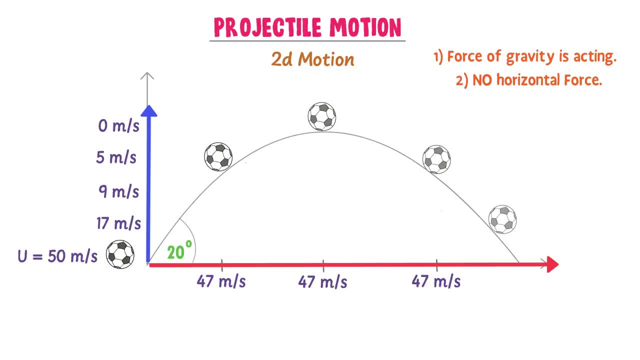 projectile or the ball at each and every point, which will further strong your concepts. For example, at this point, the vertical motion of the ball is 5 m per second and its horizontal motion is 47 m per second. At maximum height, the vertical motion of the ball becomes zero, but the horizontal motion 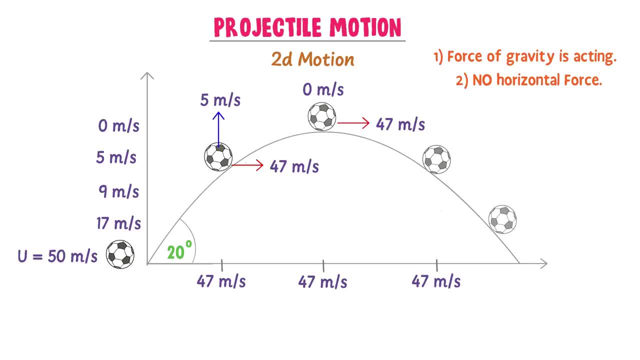 of the ball is still 47 m per second. Remember that at maximum height the motion of the ball is not zero, because the ball still moves with 47 m per second in horizontal direction. Only the y-component, or vertical component, of motion is zero. Now the ball will start falling down At this point. 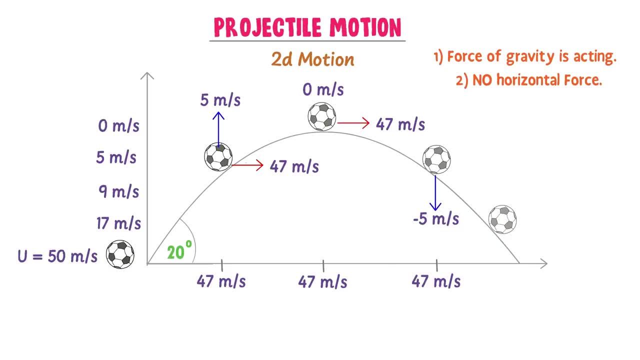 the vertical velocity of the ball is negative 5 m per second and its horizontal velocity is 47 m per second. At this point, the vertical velocity of the ball is negative 17 m per second and its horizontal velocity is 47 m per second. Remember that negative sign doesn't indicate the 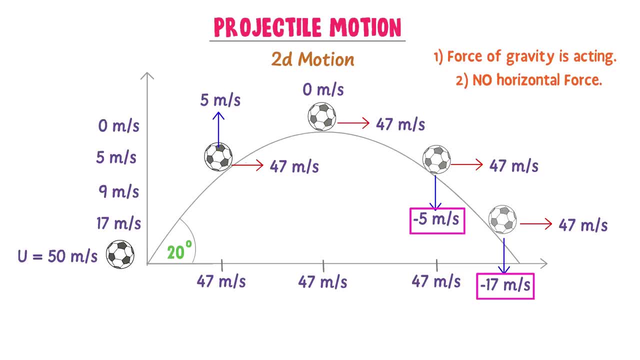 smaller value. it only indicates the opposite direction of the ball. Thus we can analyze that as the ball moves upward, its velocity decreases with the passage of time in vertical direction, But its velocity in horizontal direction remains constant At maximum height. the y-component of the 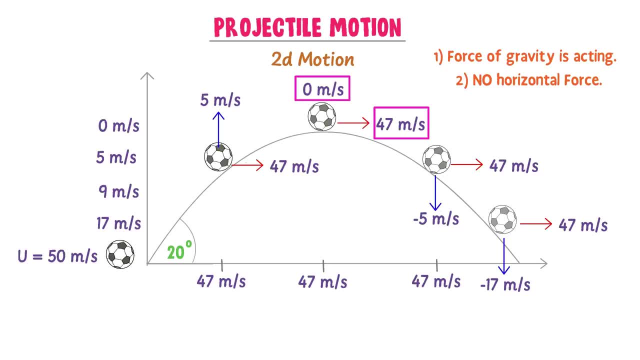 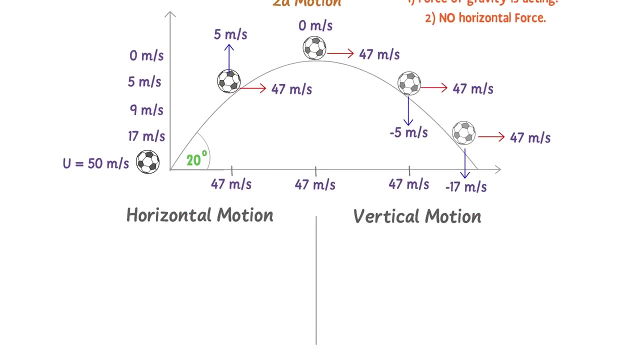 velocity is zero, but not the x-component. Secondly, when the ball falls down, its vertical motion increases with the passage of time, but its horizontal motion again remains constant. To conclude, the horizontal motion and vertical motion of the ball are projectile. We learn that.